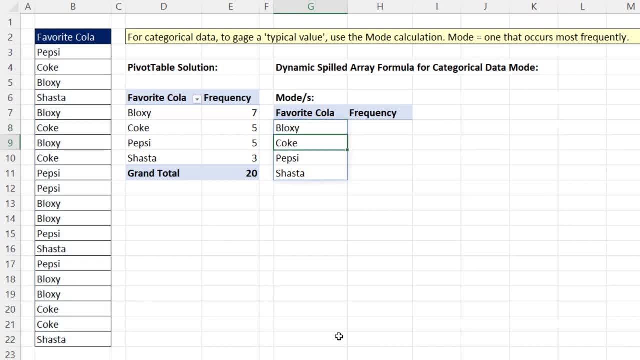 So we'll see if unique list actually spills- and it does At the top F2,. the next variable will be frequency, So I'll use F comma. The input for that variable, COUNTIFS Criteria range, is the full column C. 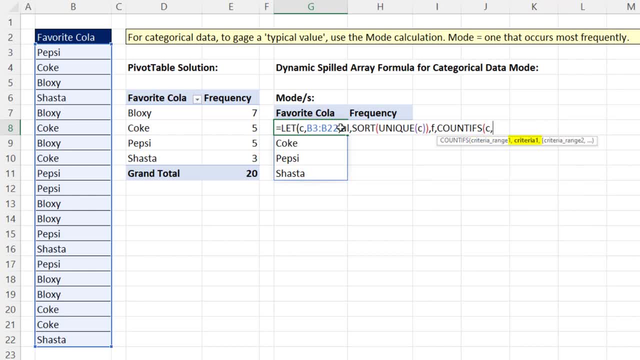 Comma, and in Criteria 1, we need the criteria for counting. So we'll put the unique list And that way COUNTIFS will give us a count for each item in the unique list. Close parentheses and there you go. 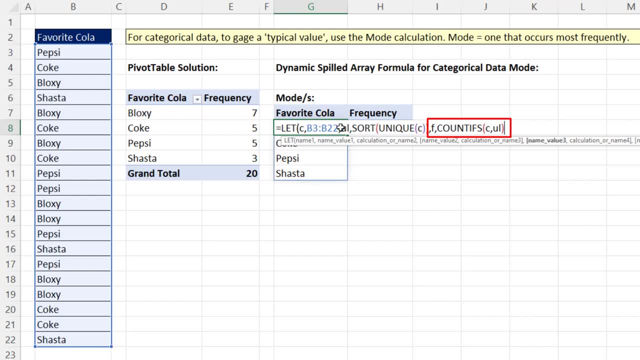 There's the third variable name, the third variable formula element, And now let's see what it evaluates to Comma F to check it. and there's the frequencies in the top cell F2.. Backspace, the next variable. 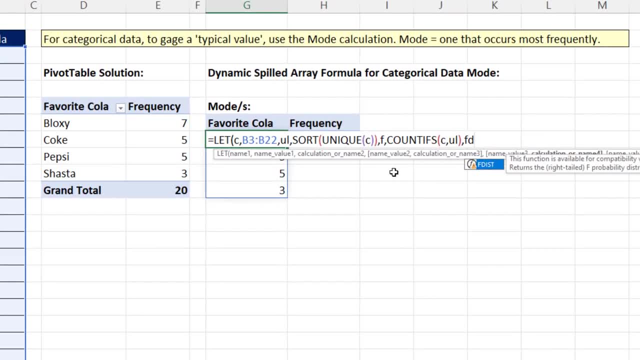 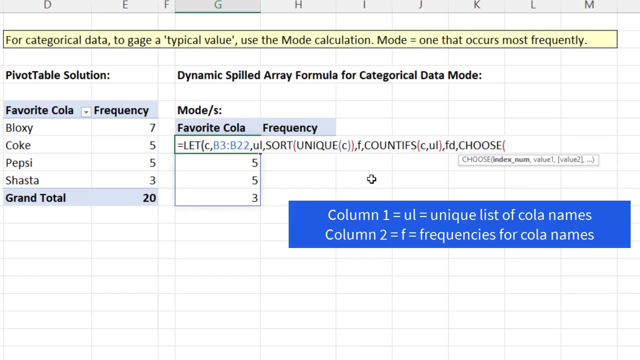 So we'll be FD for full frequency distribution comma And I'll use the LOOKUP function CHOOSE. I want to mash together two columns, so I simultaneously have to look up column 1 and 2. And you do that in ERASE syntax, column 1.. 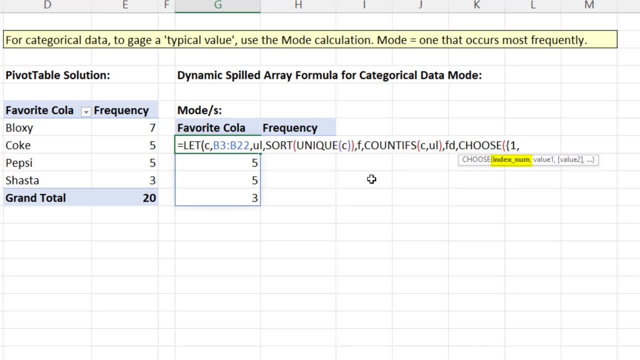 And you've got to use a comma because comma represents go over a column 2, close curly bracket. That 1 and 2 in INDEX will tell CHOOSE to look up value 1. And value 2. And return them both comma. 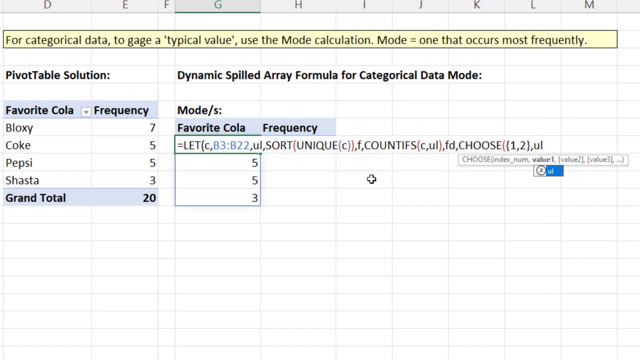 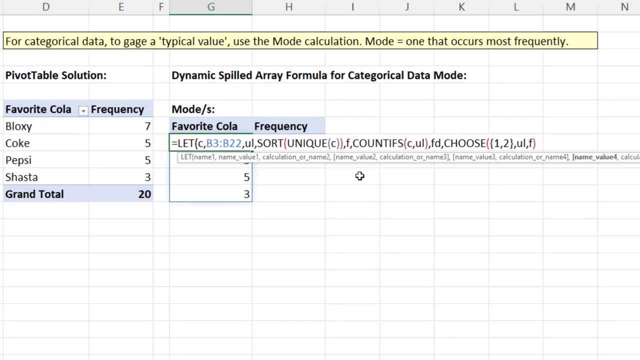 The first thing that I want to look up is unique list comma. The second thing I want to look up is frequency, And CHOOSE will look those both up and deliver them as a single object. And now we've defined the fourth variable and the fourth element for that variable. 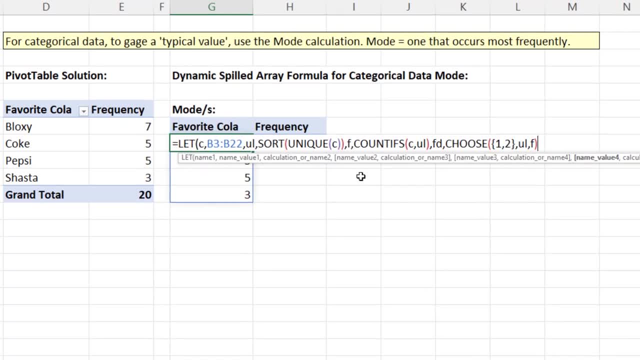 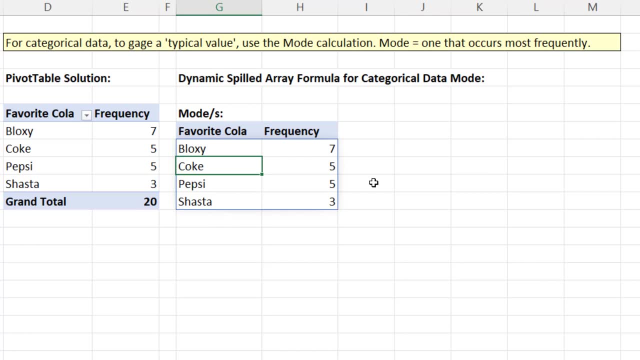 Now let's see if the frequency distribution works. So, comma and we'll check it. FD, close parentheses And ENTER. Now I have what I want. I have a table that I can filter based on the max value. So in the top cell, F2.. 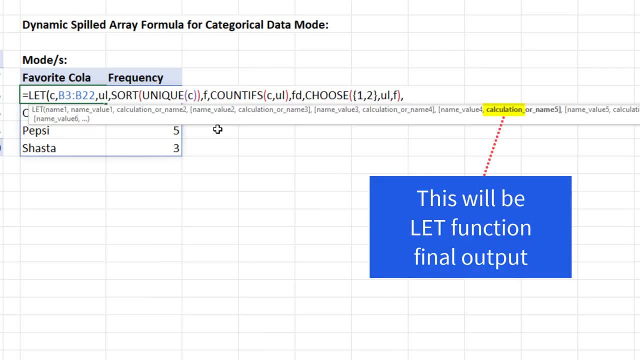 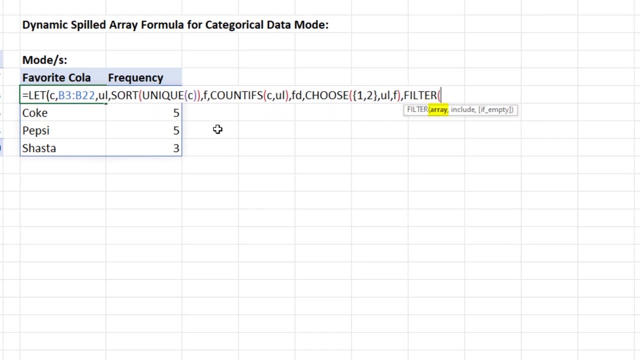 And I'm going to BACKSPACE And this is not going to be a variable name and a variable input. This will be the final calculation, So I'll use FILTER. I'm going to filter FD comma And how am I going to filter it? 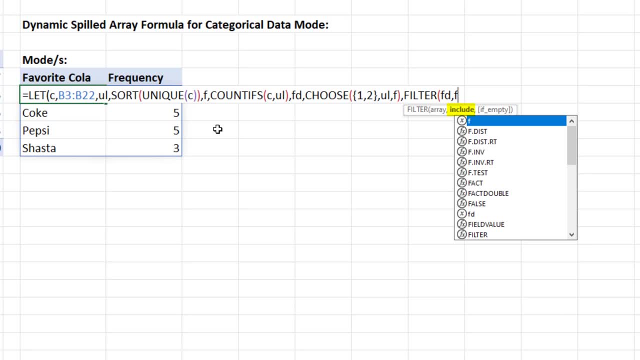 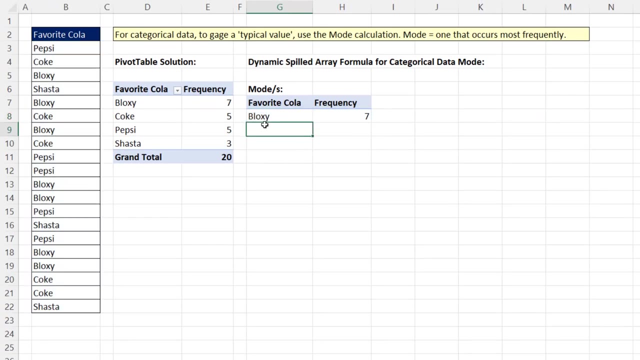 I need to look through the full spilled frequency column And say: whenever you are equal to the max frequency, Close parentheses, Close, close And ENTER. I have looked up the actual categorical label and the mode. Now, if I come over and change this to Coke, it'll meet both conditions that I set up up front. 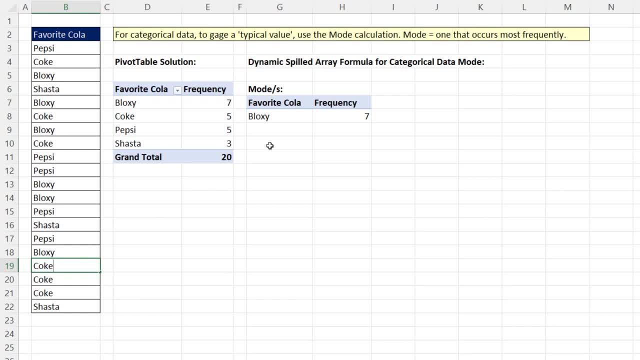 I need to be able to change the data, have it update instantly and I want everything to spill, So when I hit ENTER. that is some magic that I have been looking for for decades. And now in Microsoft 365, and all of these functions actually work in Excel 2021,. there it is. 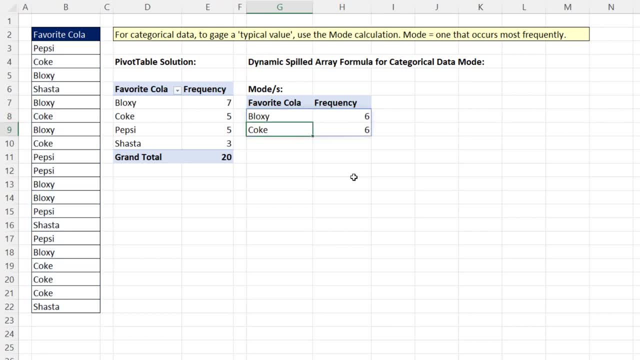 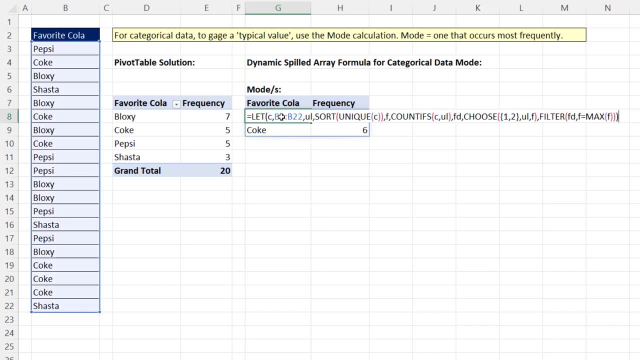 Multiple modes with categorical data, No problem. Now, I was having so much fun building this awesome new formula, I forgot what our teammate RECALC, or DI, always says: Hey, when we do a long formula like this, let's use ALT-ENTER. 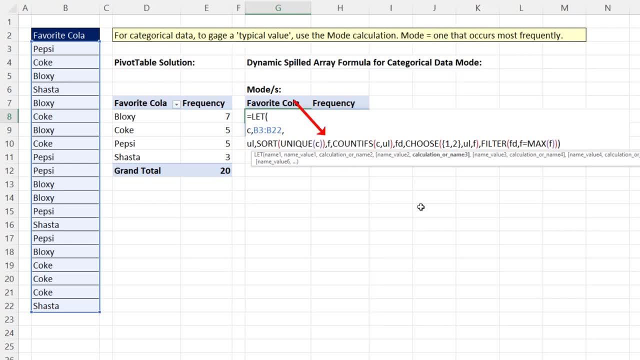 And we'll show each variable. here we go on a new line. Look at this. I'm going to put FD down to the next line And there's the final calculation, BAM On its own line. And so when I hit ENTER, it looks the same. 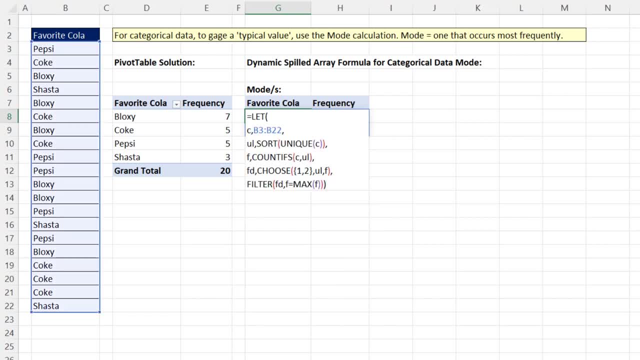 But when I come to the top cell and hit F2, that's easier to read. Well, at least for me, At least for some people, I still like it linearly, But guess what? This is an amazing formula that points towards the future. 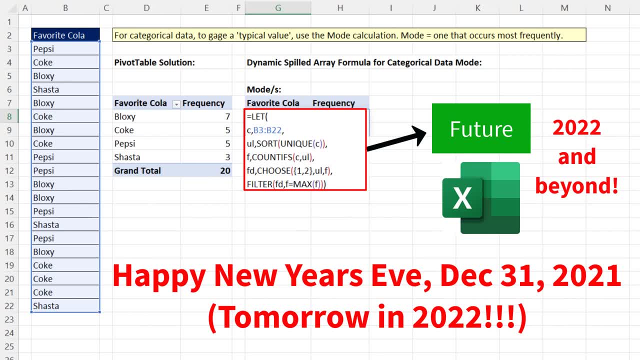 And on this New Year's Eve, on the precipice of 2022, happy and excellent New Year to you. Hey, we'll see you next year for lots more fun and lots more videos from. Excel Is Fun, All right, we'll see you next video. Bye-bye, Bye-bye.